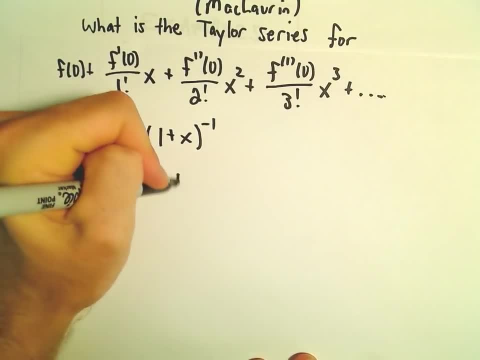 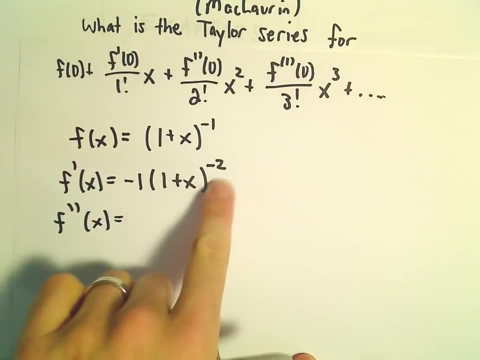 So let's see our derivative. I guess we would get negative 1 times 1 plus x to the negative. second, Our second derivative: let's see: we would have positive 2 times 1 plus x to the negative 3.. 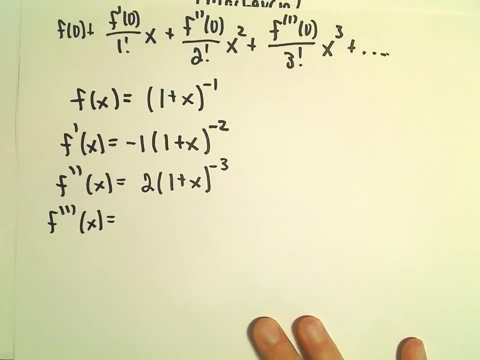 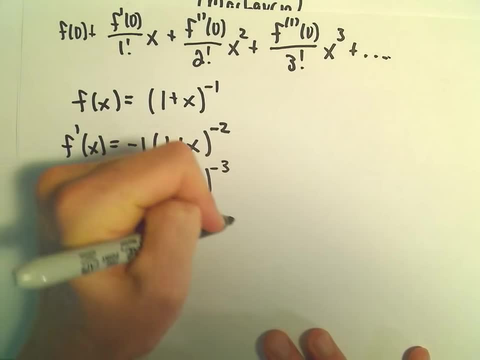 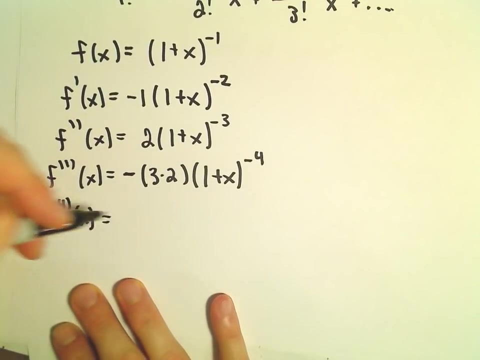 Our third derivative. we could multiply this out, but I'm not going to. We would have a negative notice. we would have 3 times 2, and then we would have 1 plus x to the negative 4th. Then I'm going to do at least one more. so the fourth derivative: we would now have a positive. 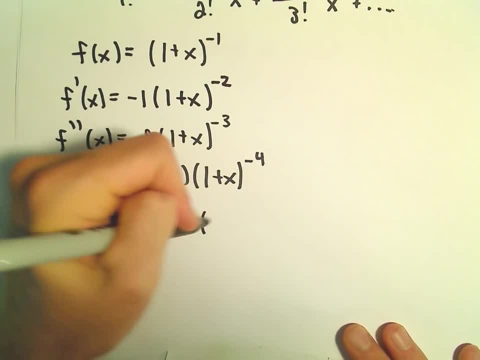 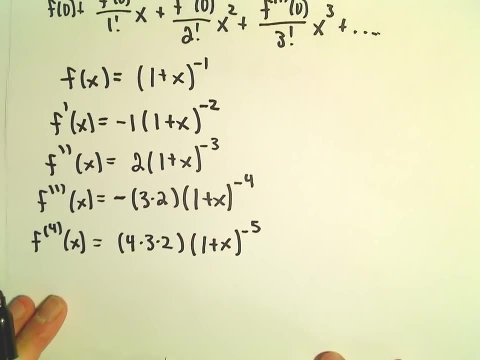 but then we would have 4 times x to the negative 4th, 3 times 3 times 2, and then 1 plus x to the negative 5th, etc. So a lot of times I don't multiply things out, just because I think it's a little bit easier to see a pattern. 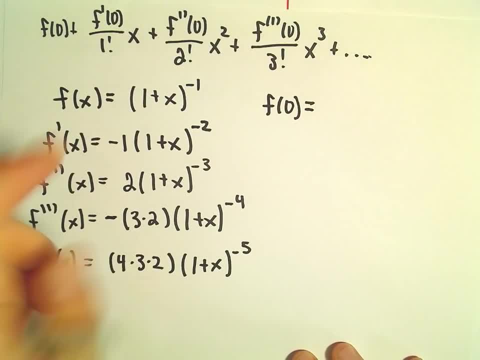 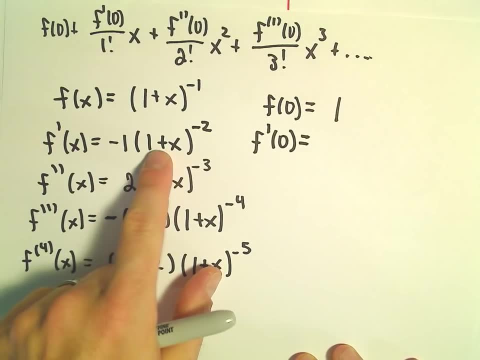 So all right, well, let's plug in our numbers. So f of 0, we'll just get 1 to the negative first, which is 1.. f, prime of 0, again we'll get 1 to. you know, in the parentheses we're going to get 1 to an exponent. 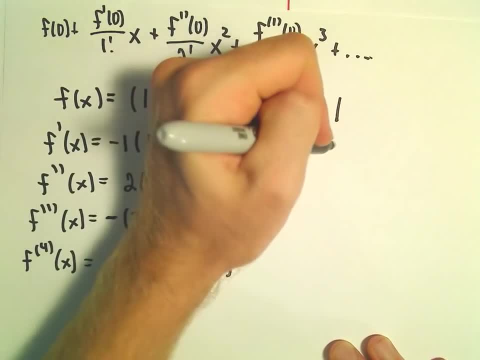 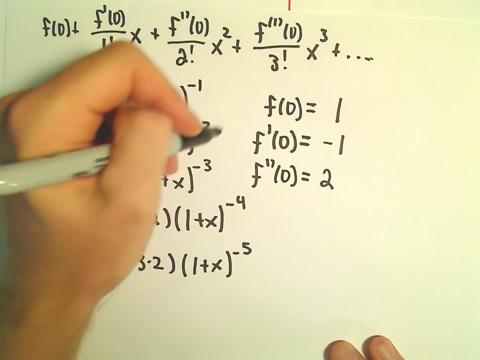 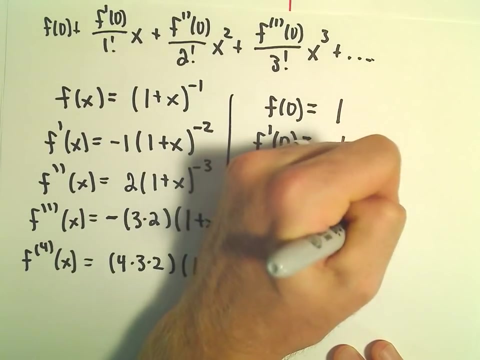 but 1 to any exponent is just 1.. So what we're going to be left with are the coefficients. So we'll get negative 1.. f- double prime of 0, that's going to be positive. 2.. f- triple prime of 0, that's going to be negative 3 times 2.. 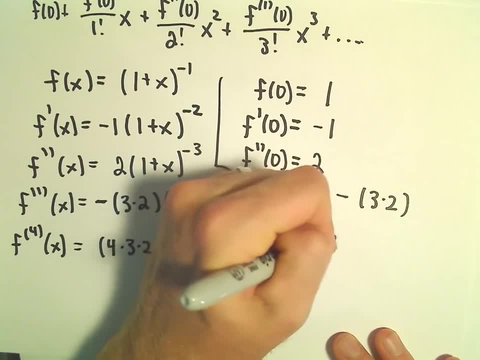 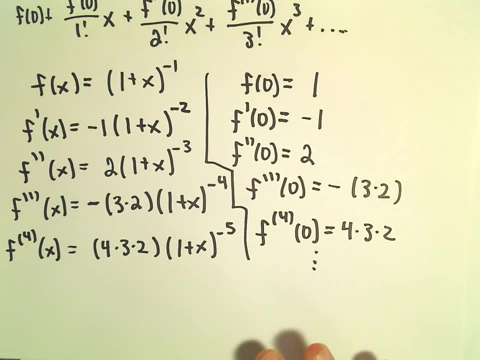 And then the fourth derivative at 0, it looks like we'll have positive 4 times, 3 times 2, etc. So the reason why I don't multiply things out is, you know, it looks like to me we're getting things involving factorials right. 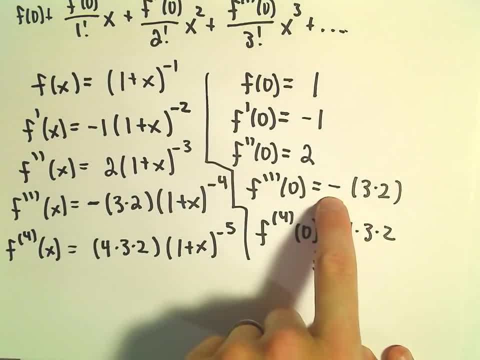 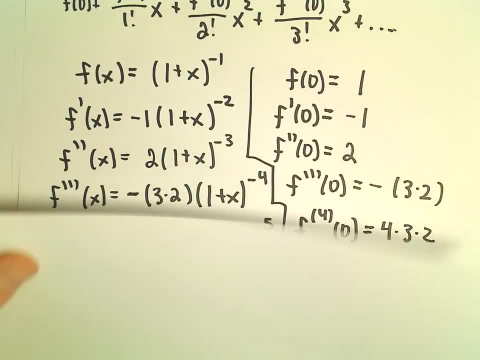 So this is 4 factorial. 3 factorial: Yeah, there's a negative in there, but we can deal with that. 2 factorial- The next one: we would get a 5 factorial. So let's see if we start filling in our formula. it says f of 0 would be 1.. 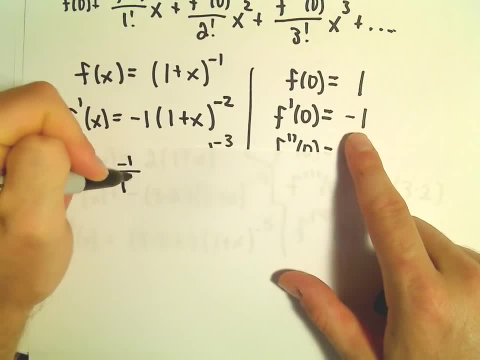 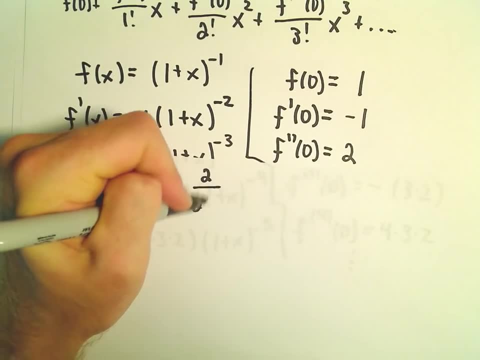 Then we would have f prime of 0, which is negative, 1 over 1 factorial times x. Let's see f double prime of 0, that's going to be 2 over 2 factorial x squared. And then let's see we would have, plus f triple prime of 0..